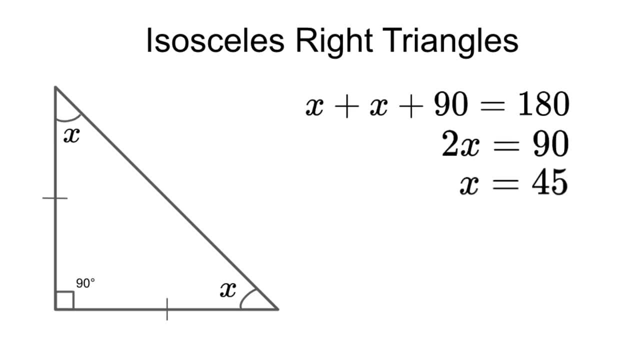 180 degrees and we calculate that each angle equals to 45 degrees. Let's now try to find out the relation between legs and the hypotenuse. Let's call the equal sides of a triangle as A and try to find out the hypotenuse of the triangle. We will use the Pythagorean. 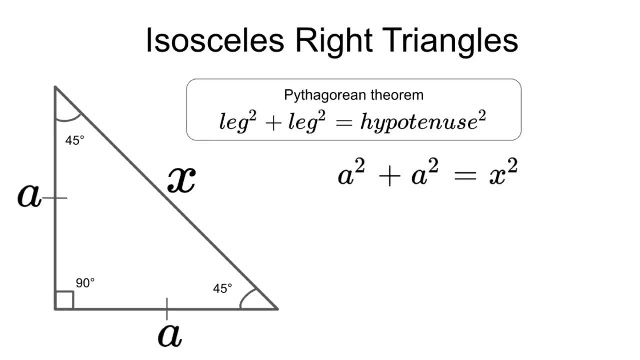 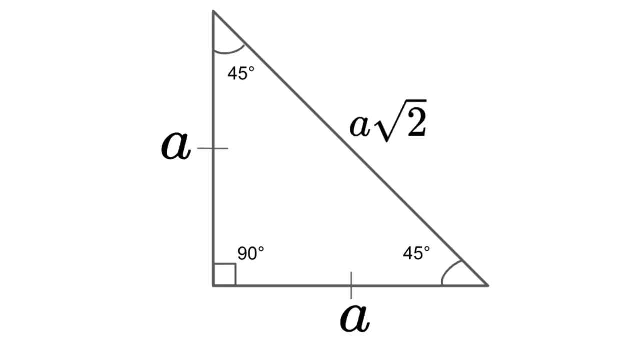 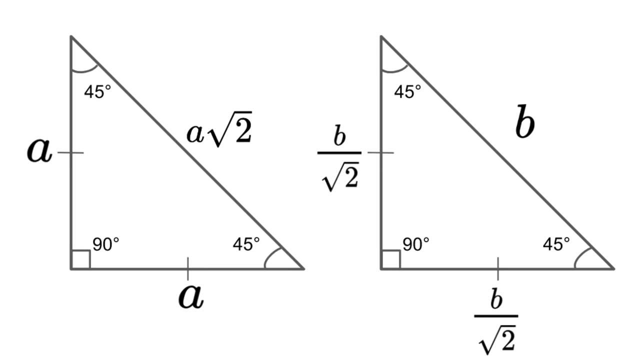 theorem And here we will have: A squared plus A squared equals to X squared, And through calculations we will find out that X equals to A multiplied square root of 2.. Also, we can rewrite it in a different way: If the hypotenuse would be B, then each other side would be B divided. 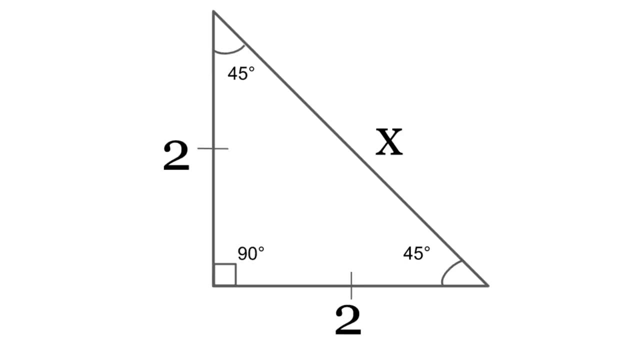 by square root of 2.. Let's have some practice now. Here we have 2 and 2 as the sides of the triangle and we need to find out the hypotenuse. Then the X will be equal to 2 multiplied square root of 2 or 2 square root of 2.. Next here: 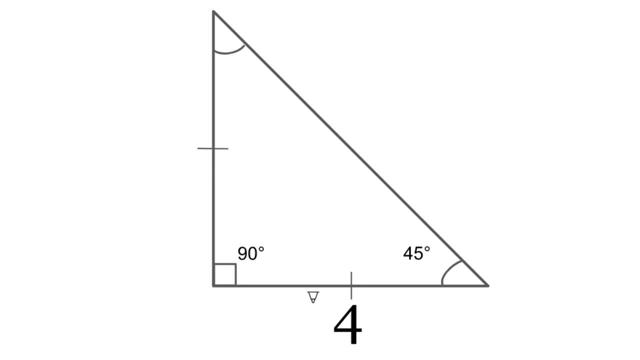 we also have just one side of the right triangle. We know that this is also will be 45 degrees and this side also will be 45 degrees. So we have 2 and 2 as the sides of the triangle, So it's also will be 4 and if this part, dehydration would be, would be 4 multiplied square root. 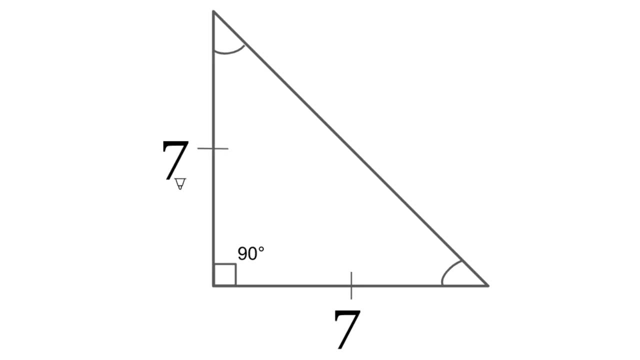 of 2.. So again, the degrees will be 45 and the hypotenuse would be seven multiplied by square root of 2.. And here we have hypotenuses And we need to find out the other sides of the right triangle. 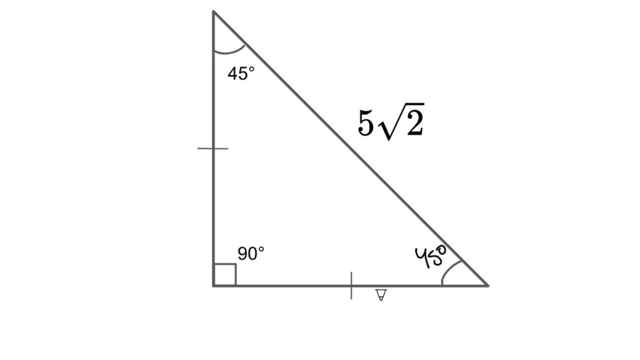 This is also going to the edge. it is also going to be merged respectively: Come on, just shoot your hand, tu Bijuuu And ride ash anybody. do you think that it works out? mike be 45 degrees and each side would be 5 square root of 2 divided by square root of 2, and this: